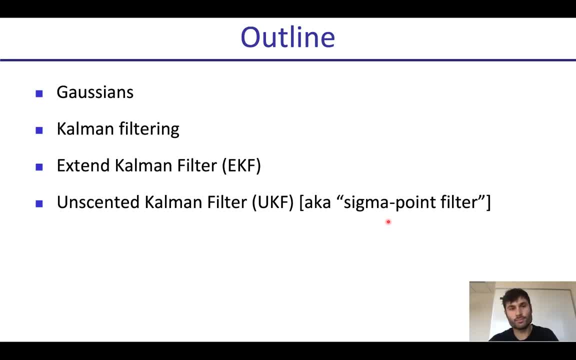 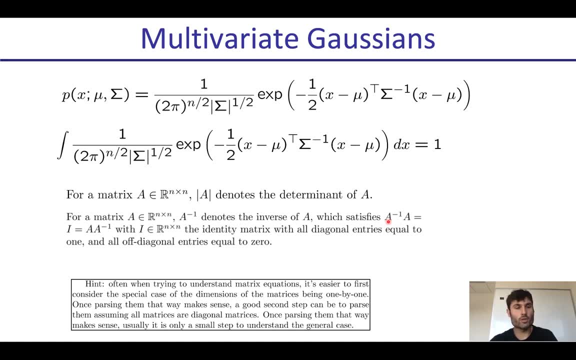 Kalman filter, also known as sigma point filter. So let's first talk about the multivariate Gaussian. So a multivariate Gaussian is defined by two parameters: One is a vector, mu, and the other one is a matrix sigma. This equation on the top is the definition of the of the pdf of multivariate Gaussian. 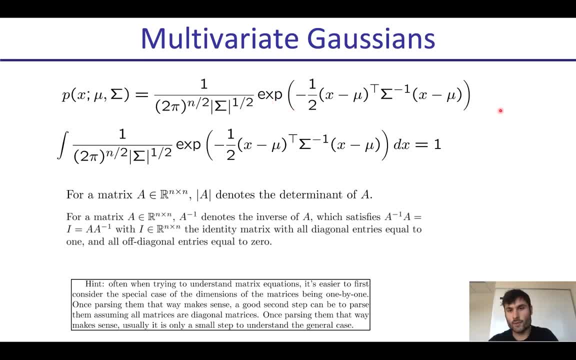 And it's essentially defined by this term of the exponential. So essentially, multivariate Gaussian is defined by being the quadratic, like the exponential of a quadratic, And we see that the parameter mu acts as a location parameter, It actually just centers the pdf And the sigma parameter acts as a scale parameter. 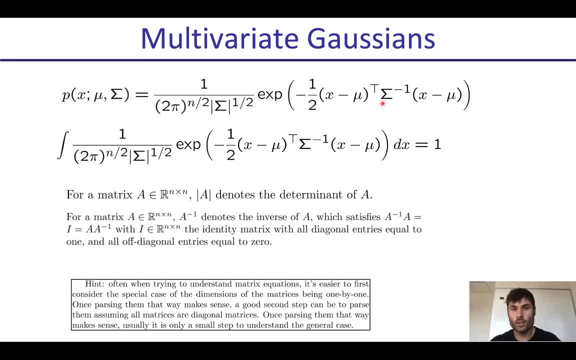 This sigma, this matrix, cannot be whatever matrix. It has to satisfy three conditions: The first one is that it needs to be symmetrical, The second one is that it needs to be positive, definite, And the third one is that the inverse needs to exist, because 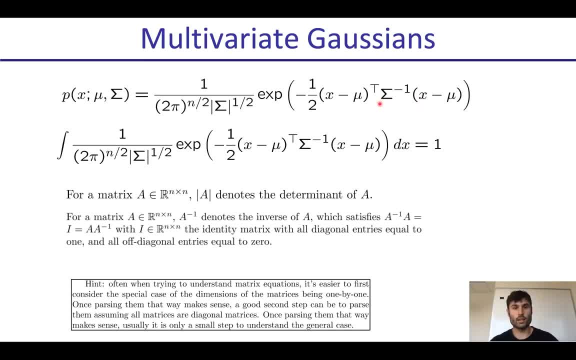 we need to take the inverse here, So we don't want this to be ill-defined. The other term of the pdf, these scalar terms here that depends on pi, the dimension n and the determinant of the matrix sigma simply acts as a normalization constant. So 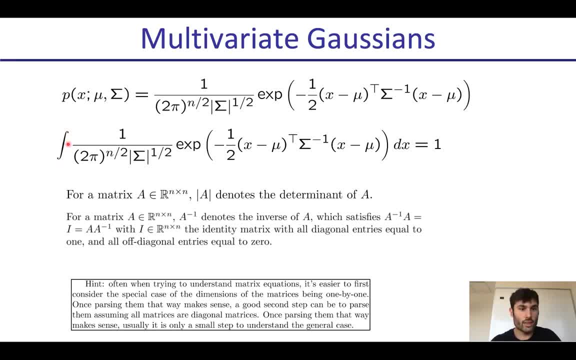 thanks to this term over here we have the integral over all possible axes It's equals to one. So this relationship will be pretty important in the lecture. so this means that the integral of these exponential is exponential terms. it's equal to the term in the denominator. 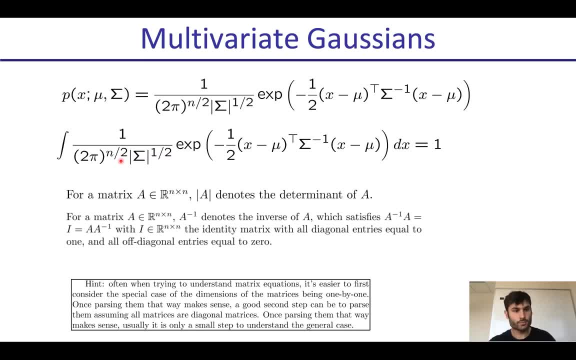 and we will use these a little further on. Let's look for some quick notation. Given a matrix—a, Whenever we write down the a between bars, it denotes that it's the determinant of this matrix. And then, when we see a to the power of minus 1, since, like here and here, it denotes the inverse of this matrix. So 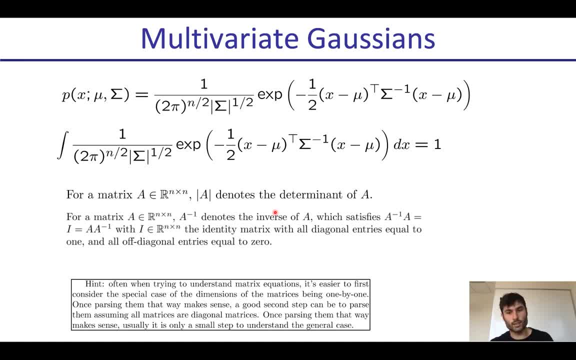 essentially, it satisfies the inverse, satisfies that the a to the power of minus 1 times a is equal to identity and a times the times a to the power of minus 1, it's equal to the identity as well. And for all these equations and formulas, it's pretty. it's usually easier if you think of: 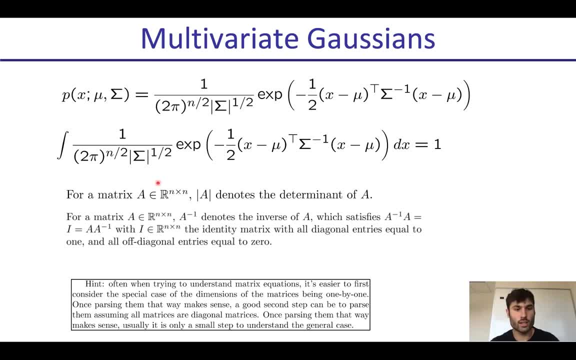 it in the one-dimensional case. So, essentially, instead of these metrics being n by n, just think of it as being one by one, which essentially means that this scalar, which is the case of the univariate Gaussian variable, we have in the one by one case. 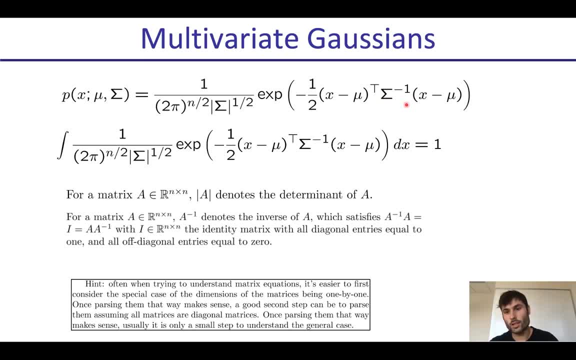 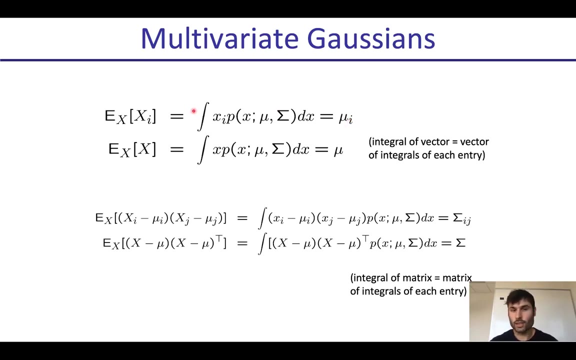 we have: sigma is equal to the square of the lowercase sigma. and then we have this x minus mu transpose times: x minus mu is simply x minus mu squared. So essentially, we have essentially obtained the same PDF as in the univariate case. Now we will explain what all of this mu and sigma. 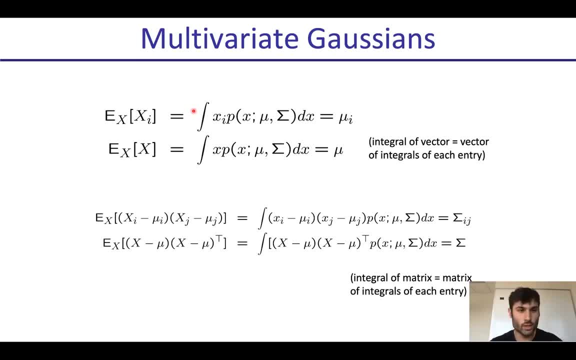 parameters mean. Probably all of you will have like imagine of the mu i. mu i is the ith component of the parameter. mu refers to the expectation of the random variable x, the ith component of the random variable x. So essentially, if you do the expectation of x i, you end up obtaining the mu i. 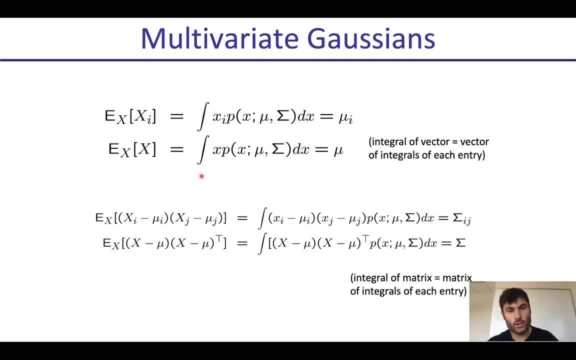 And then here we have the vector notation, where the internal of this vector x with respect to the PDF, essentially means that taking the scalar integral, so the integral that probably all of you are used to do, for each of the dimensions, And this extends the same to the matrix case. So if we compute the matrix sigma, 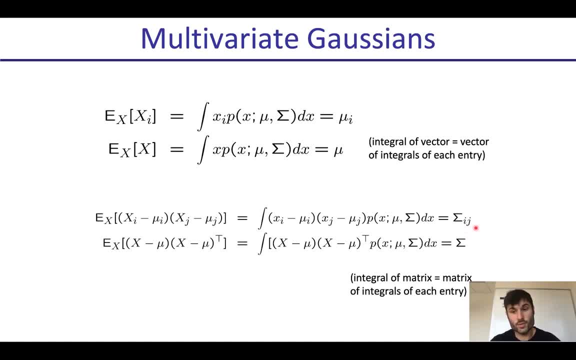 essentially the component ij, it's the covariance, so it's the ij covariance of the covariance matrix And we can say, because this essentially is the definition of the covariance, so x i minus mu i, times x j minus mu j, if you take the expectation of this multiplication, 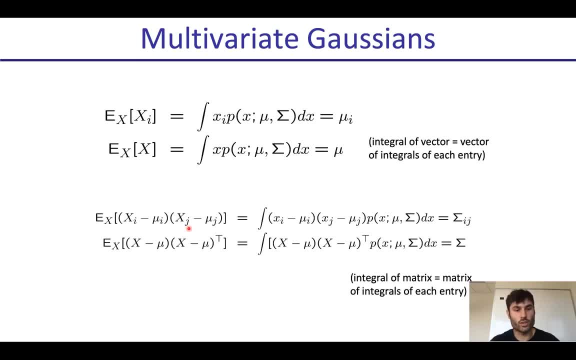 essentially, this is the covariance between these two random variables And if we do the integral of that, we end up obtaining that this is the ij component of the covariance matrix And in the vector notation, or matrix notation in this case, what this interval means is just doing the interval for each of the components of the matrix. 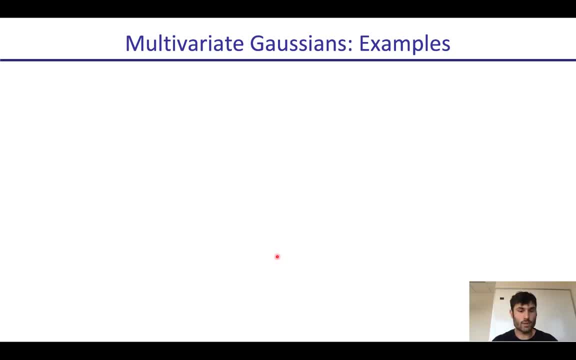 Okay, now we'll see some examples of how these parameters affect the underlying PDF. So here we have a Gaussian distribution data center around 1, 0.. So we see that in this, in the first axis, the mean, the mu, is centered in the value of 1,. 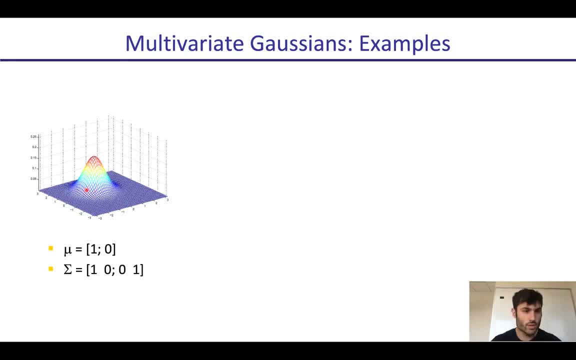 and then the second axis is centered at the value of 0. So we have this d-shape around the value 1, 0. And then we have a diagonal, a diagonal covariance. that's essentially the identity matrix. So if we move the, if we change the parameter mu, essentially what we have is we just move the. 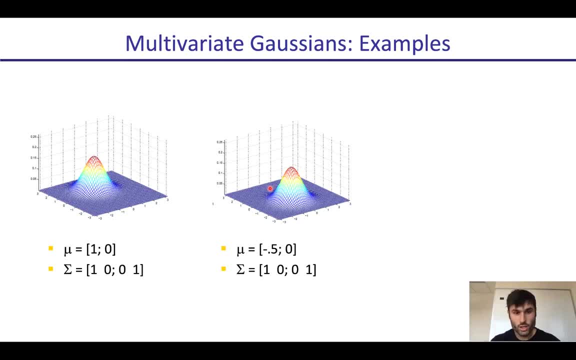 entire, the entire function to be centered at an around another point. So right now this is centered around the point minus 0.5 and 0. And we can just keep shifting this around by just changing the parameter mu. That's why I say before the mu acts as a location parameter. 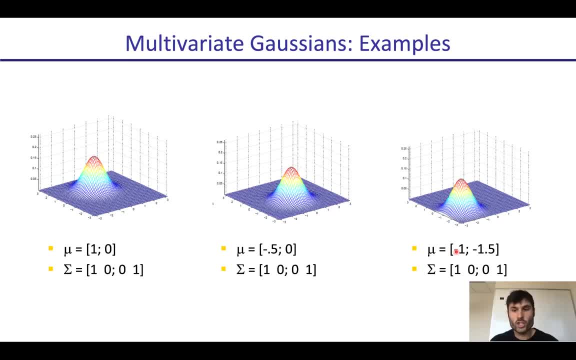 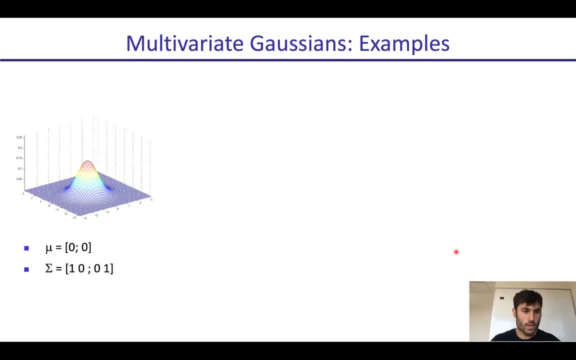 So because it's just preserving the shape but just moving the entire distribution around. So now we play what happens if we change the covariance matrix. So here in this function we have just kept the mu the same, but we have just scaled the covariance matrix. In this case, 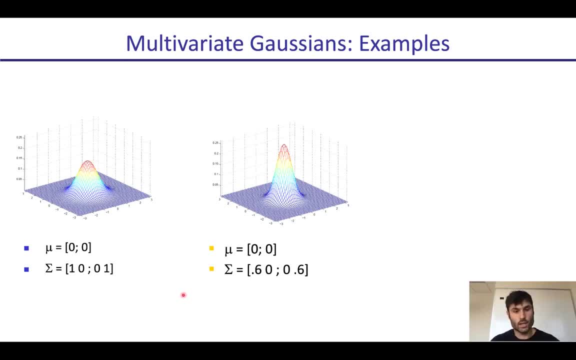 we have shrinked it. So now, instead of having values, the identity, the only terms to be 1, 1,, it's 0.6, 0.6.. And what this results is that this new random variable has less variance. 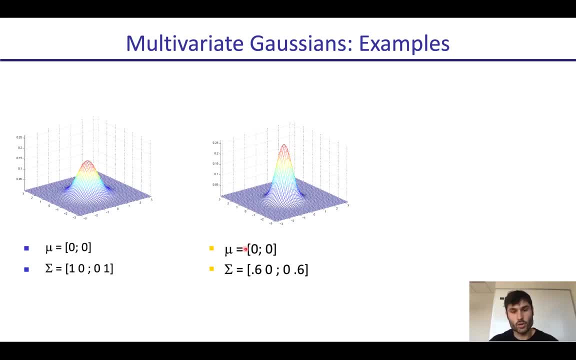 So all the mass is centered around mu, And what this means is, like it has. the PDF has higher value on mu and then nearby points compared with the identity covariance, And instead of what we do is shrinking the covariance matrix, we just make it larger. What we end up having is that the points around the mean have actually 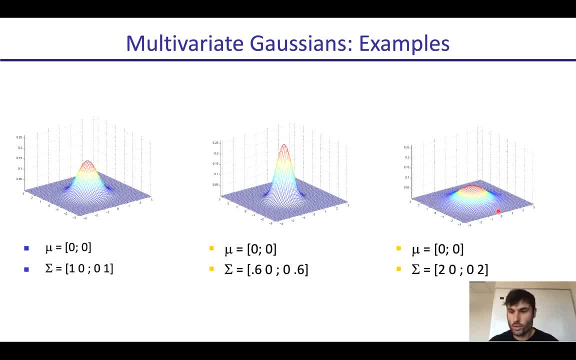 have a lower value than the previous ones, But the points that are further away from the mean have a slightly higher value, And the reason why is that when it has these different heights is because it has to integrate to one. So if you make the points farther apart to have a larger, 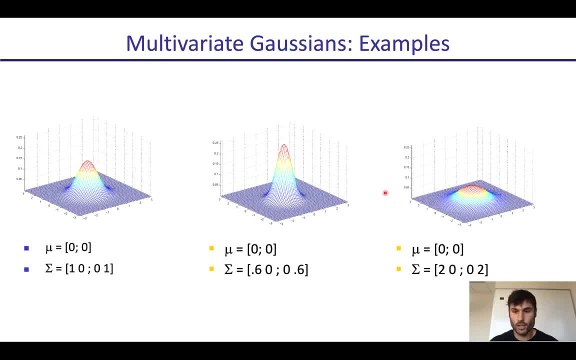 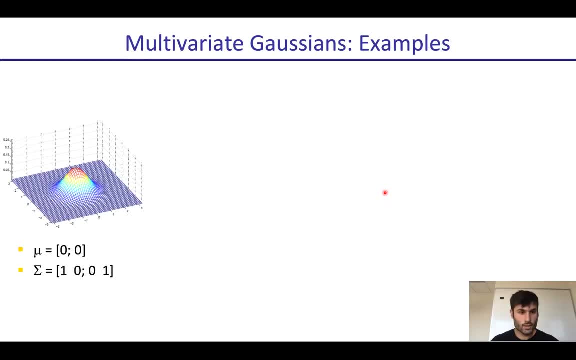 mass. that will contribute to the points that are around the mean to have lower mass. So now we'll consider the cases where the covariance is not diagonal but it has off. Essentially, we have a covariance matrix that is 1.5 and the second row is 0.51.. What this means is: 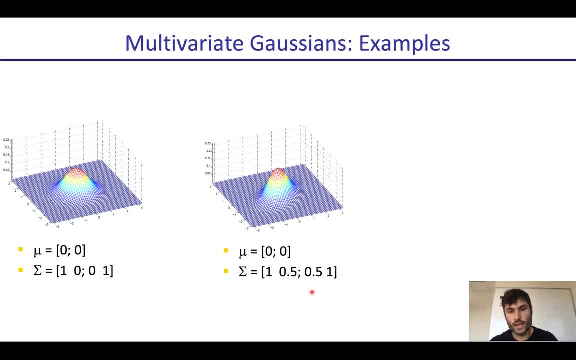 that there is a positive correlation between the first axis and the second axis, And we can see it in the shape of this distribution. So what this means is like if we increase the value of the variable x, the probability of x, of y having a higher value also increases, And that's why it has. 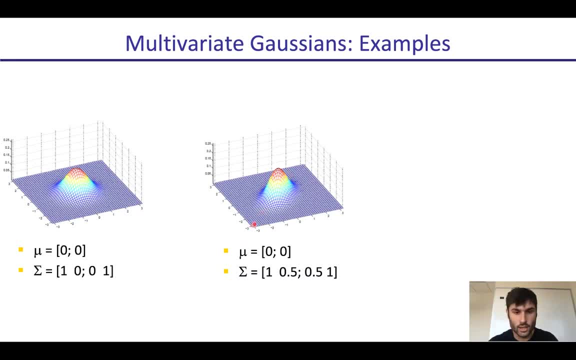 a sort of elliptical shape that is aligned to the x. x equals y. So we have this x equals y that has a trace where this ellipsoid is, one of the axes of this ellipsoid is aligned, And then we can correlate them even more by just increasing the value of this. 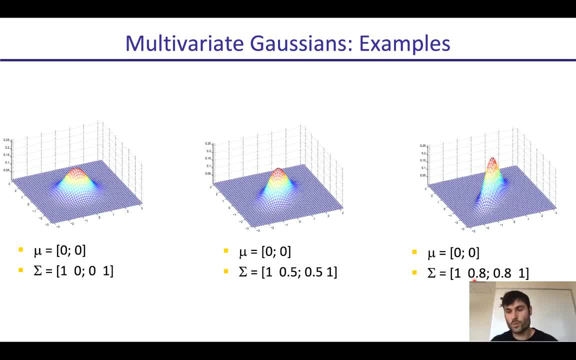 of the anal terms And the limit of this being close to one, because if it's one, then you won't have the covariance, won't be invertible. But in the limit of this being close to one, what we'll have is: 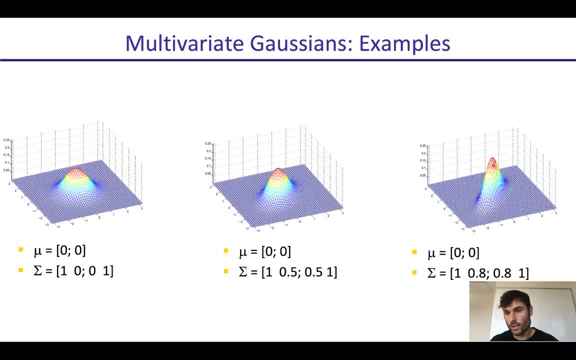 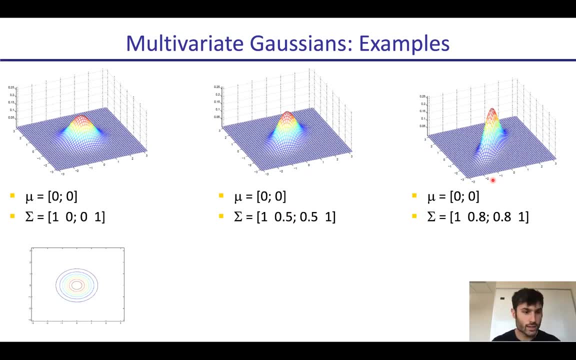 almost just one line, a very thin type shape. We can see this, what I was referring to, like the ellipsoids and the different shapes. So in the first one, we see that this is a perfect circle where there is no misalignment of the axis. However, in this case, since there is, 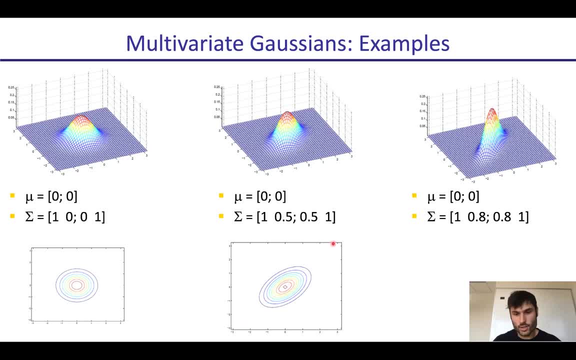 correlation between x and y. we see that there is one of the axes of the ellipsoid. is this: y equals x, term this like diagonal line, And here we see that this is even this is this is the distinction, or this axis is even more sharp. 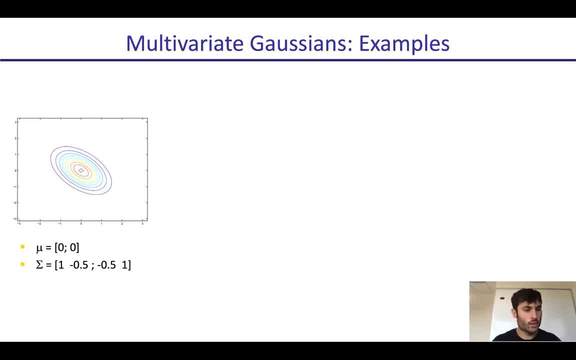 Here we have other cases in this, in this 2D, 2D contours, And we can also have correlations that are negative. So here we have: if the value of the y axis increases, actually it's more likely for the, for the x to be to be negative. And we have even stronger correlations when 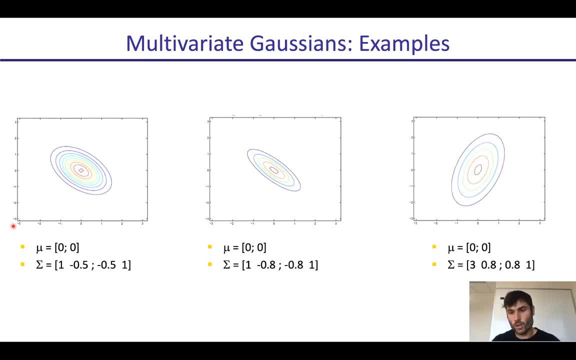 correlations are negative And also we can have cases where the, the, the diagonal torus, doesn't have to be one, they can just be scaled up at any by any, any constant, The only conditions that, as I said before, the covariance matrix needs to satisfy. 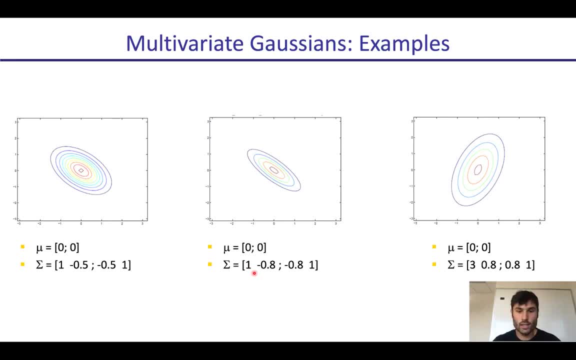 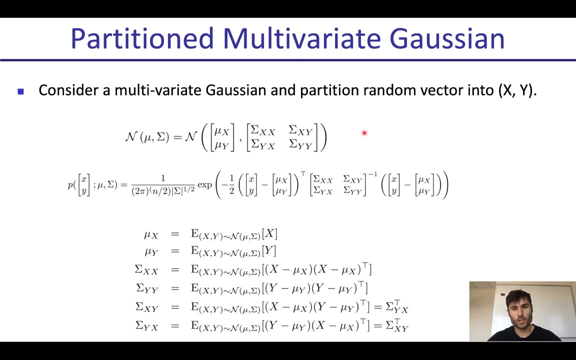 is that it's invertical, it's symmetrical and it's also a positive definite, So its eigenvalues are larger than zero. So, given a multivariate Gaussian distribution that that is high dimensional or has more than two dimensions, we want to be able to write it down instead of 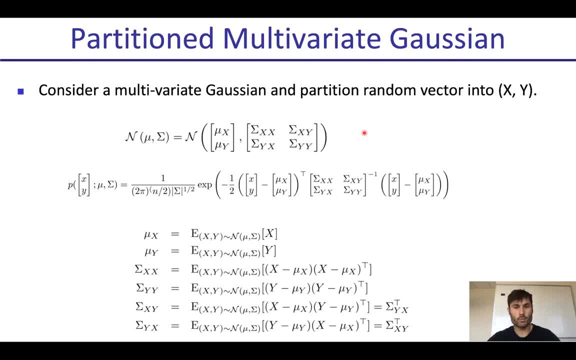 in terms of its components. So you can imagine a random vector. just split this random vector into two, into two sets. One is x and y, So the continuation of those leads to the original vector And we want to be able to write down. 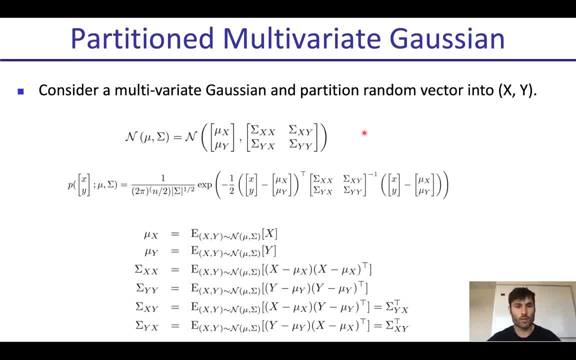 the entire vector in terms of the expectation and covariance of x and y. And why is this useful? This is useful because we will have to operate these higher dimensional vectors. We'll essentially have to do marginalization and condition of the. with respect to some entries. 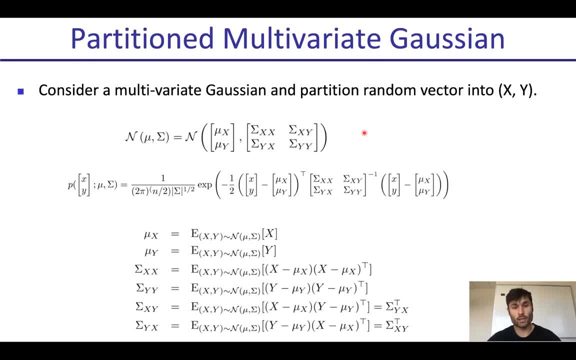 respect to some entries of the vector, so we want to be able to manipulate it in terms of the partitions. So this is pretty straightforward. we can just write down the mu and the sigma instead of like the mu x and mu y. they're respectively the mean of the vectors x and y. 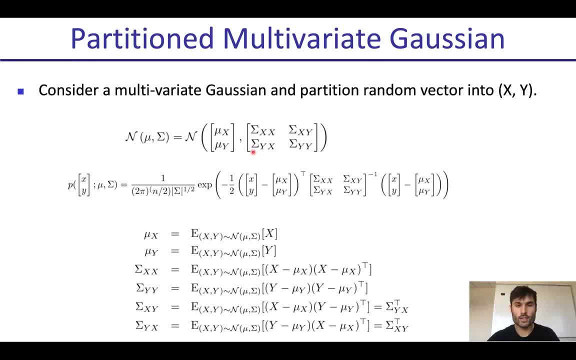 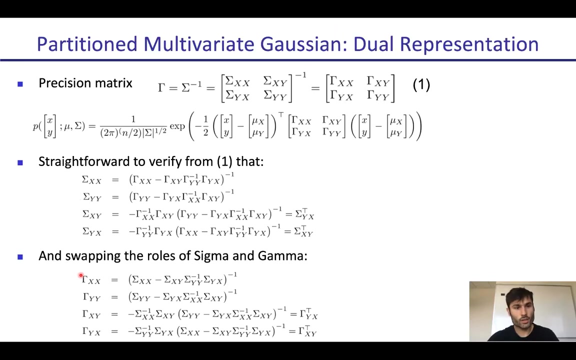 and then the covariance matrix can be written down as a block partition matrix, with which each of the entries are the covariance of x and then the covariance between x and y and the covariance of y. so here we have all the relationships, And furthermore we can have a dual view of the Gaussian variable. 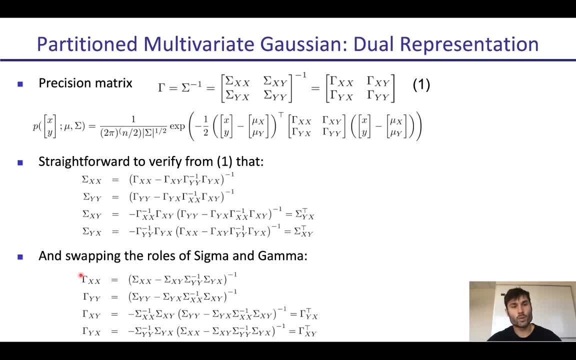 where, instead of writing into the covariance, we write it in terms of the precision matrix, that is, this is the gamma function, that is, the inverse of the covariance. And the reason why it's useful is because doing algebraic manipulations with the inverse, 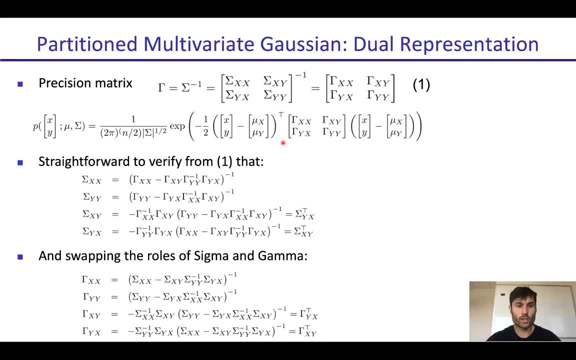 it's very tedious, so it's much more convenient if you can write down the pdf without having to deal with inverses. So now the pdf just depends on the precision matrix and it doesn't depend on the inverse of anything. So using the qualities for the inversion of block partition matrices, 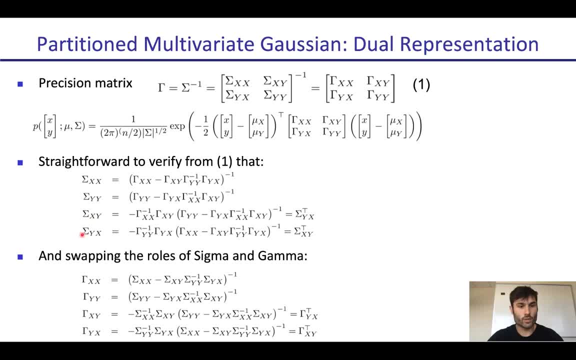 it's pretty straightforward to verify this set of relationships and I don't know if someone will notice, but this is the sure complement of the precision matrix, So this is a relationship that perspires often in algebra. And then, since the precision matrix is the inverse of the covariance, 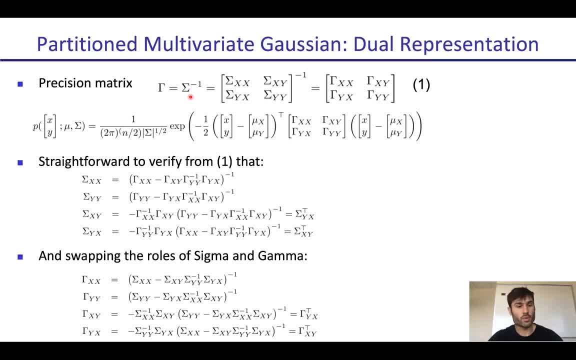 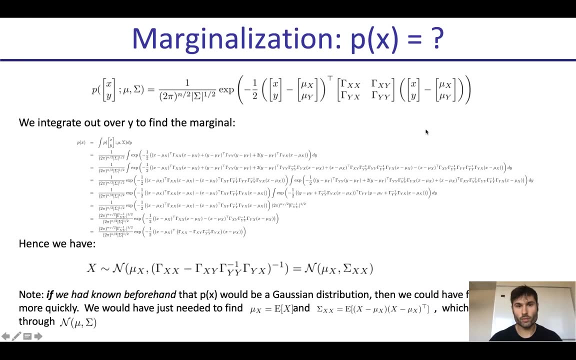 we have that the covariance is the inverse of the precision matrix. so just swapping the roles of sigma and gamma we can get the other relationships that tell you how to obtain the precision matrix with the covariance's terms. So the first operation that we'll see is the marginalization. 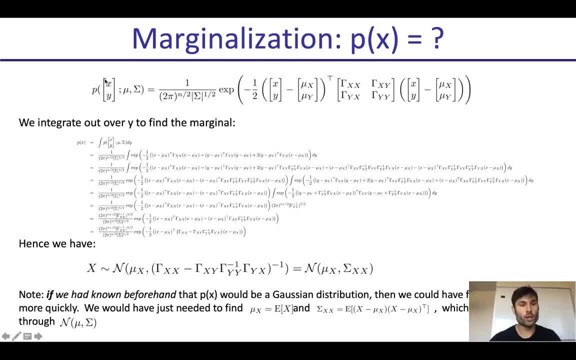 So essentially, given the joint distribution of x and y, where these define a multivariate Gaussian random variable, we want to find out the distribution of just x. So we have no idea of like what distribution whatsoever will be. So we'll do all these algebraic operations with the precision matrix because, as I said before, 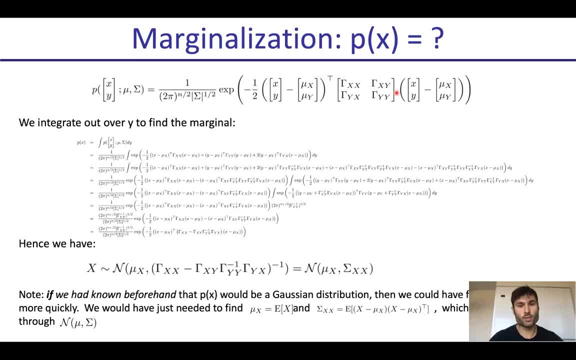 it's more convenient and easier to manipulate instead of having the inverse of the covariance here. So in order to find out what's the marginal of x, what we need to do is just integrate out the random vector y from the PDF, And this math looks pretty daunting, but we will work through it. 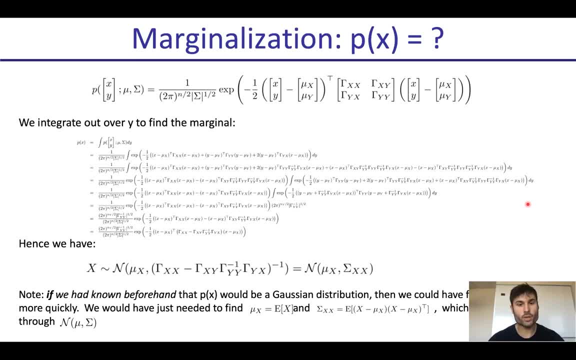 step by step And we'll see that it's like pretty straightforward to obtain the marginal of x. So the first line over here is just expanding out the PDF And we essentially discovered that we have this term over here that just depends on x, and then this term that just depends on y. 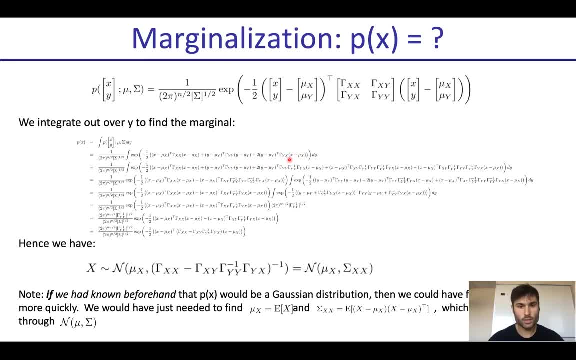 and this other term that depends on x and y. So this term that depends on x, it won't be involved at all with the integral, because it's just the integral with respect to y And then the other terms. this just depends on y and these. that depends on x and y. 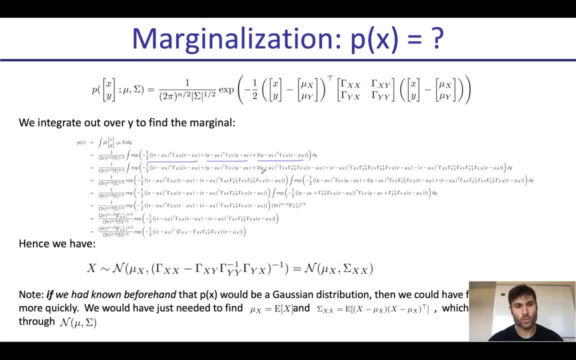 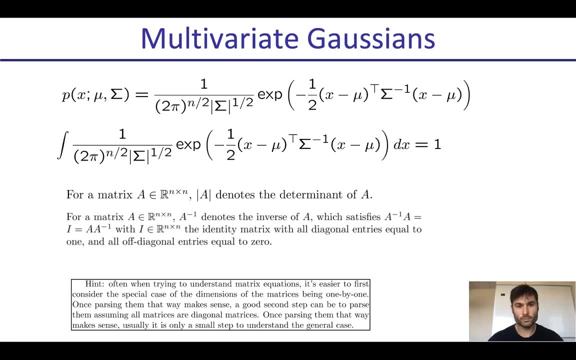 it very much resembles a quadratic And it's very hard to integrate the exponential of a quadratic. but we know from the for almost the first slide, so if we go back to it um, that if we have a quadratic of this form we know that the integral. so just moving this, 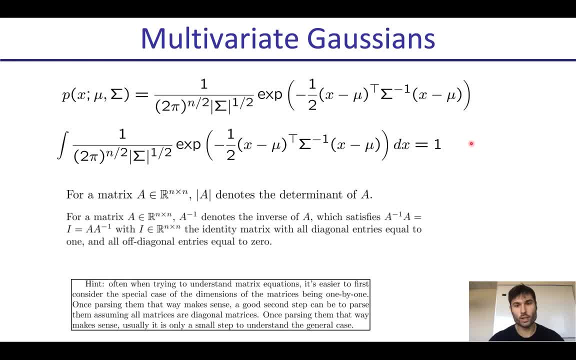 constant to the to the other side of the of the equality. we know the integral of the, this exponential- over here it's equals to these terms that involve the two pi, the dimension of the of the gaussian variable and um, and the determinant of the of the covariance matrix. 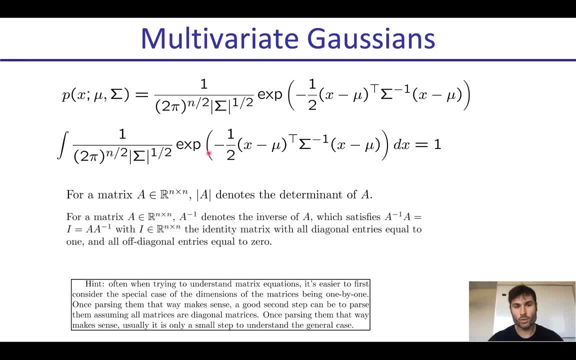 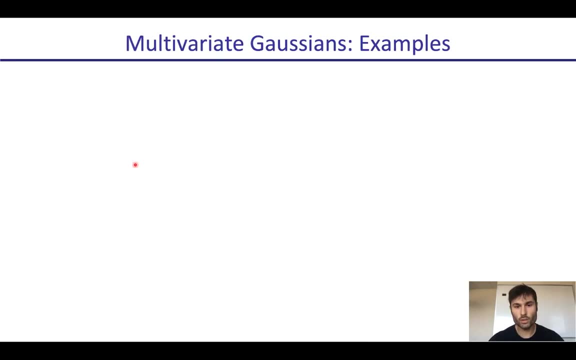 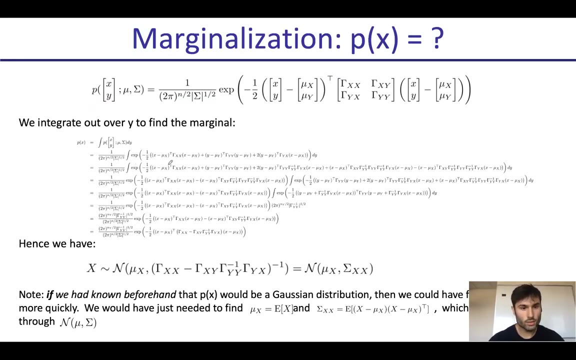 so we are able to write down the terms of the exponential uh, just like something that has this form. then we'll know what the analytic uh value of the, of the integral, so, and that's what we will try to to do in this case. so so let's say, the first term doesn't depend on y, so we'll just completely ignore it, and then 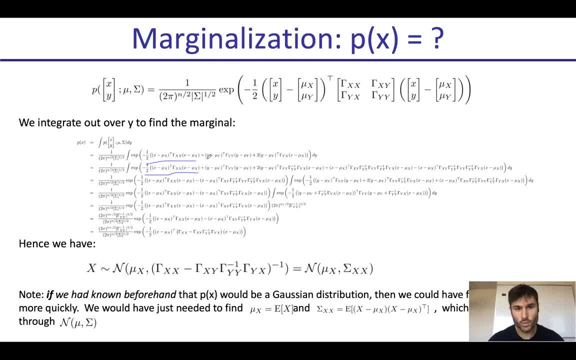 the second term. we already have some sort of a quadratic term, right, but this is not quite what we want, because there's other ways we will have. we don't know what to do with this other term over here. so these two terms will just stay as they are and essentially what we will do now is just 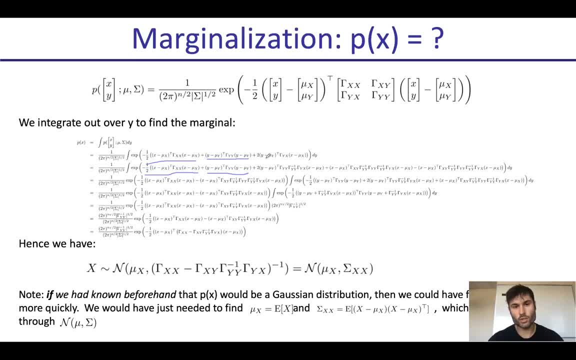 having the the, the, the completation of scores trick, but in higher dimensional. so we'll try to do the typical term of like uh, a plus b squared equals to a square, uh plus two times ab. a, b plus b square, right. so we'll try to do this in the higher dimensional term. 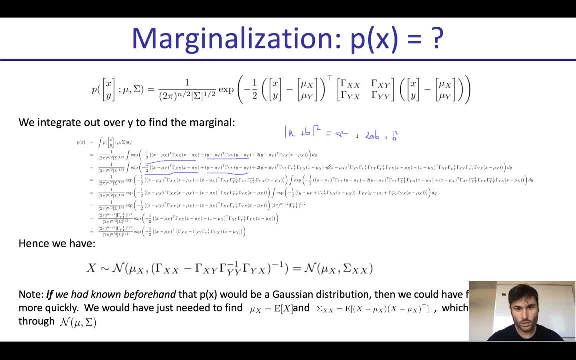 um. so here we can consider it like this: first term is the a square, and then we have to be able to write it in like two a b square, like two a b, so we already have the two here, which is nice, and then we can consider that this is like the um, this a square. so now what we can do, simply, is just: 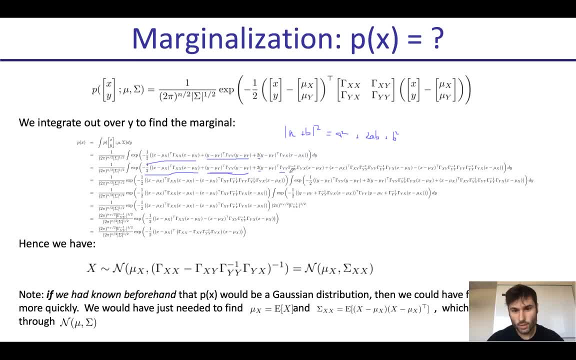 uh, add this term over here. that is doing nothing because, like gamma y y times gamma y y inverse, it just equals to one. so we have other this term. that doesn't modify at all all the equation, but they give us the the a component, right, because now we have y minus mu y times, uh, gamma y y. that is sort of like the square root of of this term. 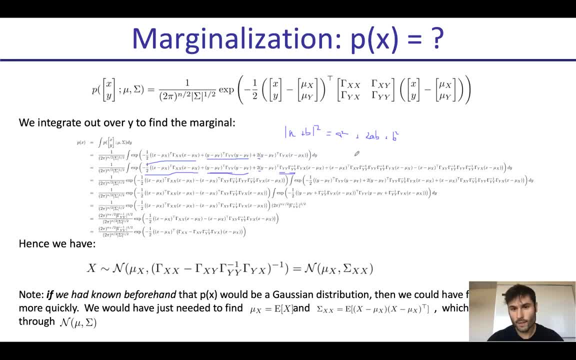 over here, and then we just need to deal now with the b term. and now we know that we see that the term is this sort of like: gamma y- y inverse times one, gamma y- x times x minus mu x. so what we do now is just add: 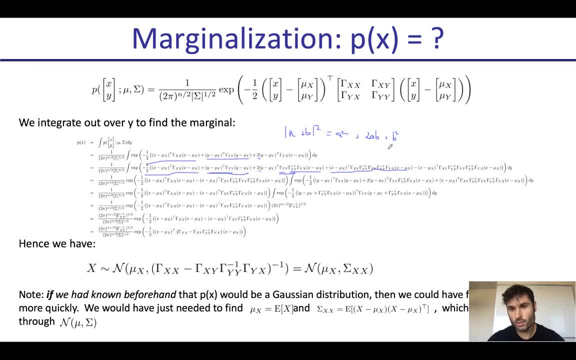 all this, this b term square, and subtract it, subtract it again. so we have modified at all this equation. the only thing that we have done is just adding this one over here in front of, like the gamma times its inverse, and then adding and subtracting this b square term. 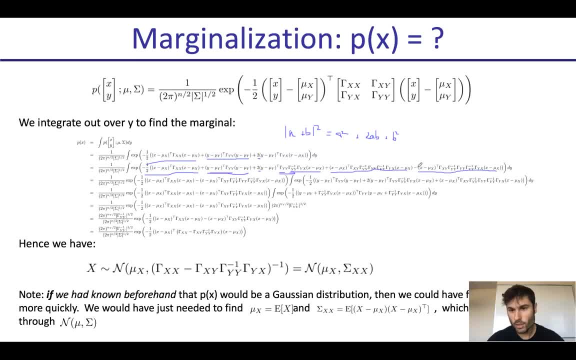 so this part over here actually just also just depends on x, so it won't be involved at all with the, with the integral. so now what we do is like just put in front all the terms that just depend on x and won't be at all affected by the integral, and then now we have this, the other terms that 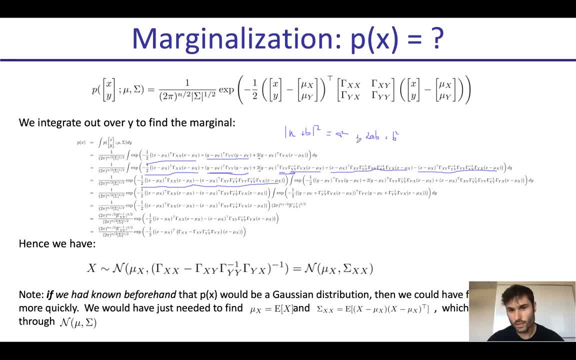 have the y involved. but this term now is like: as of this formula, it's like a square and there's like two times b, and here we have the b square, so we can just write it then as a quadratic. now, essentially, we have the form that we wanted. like that, we know what. we know what's the interior. 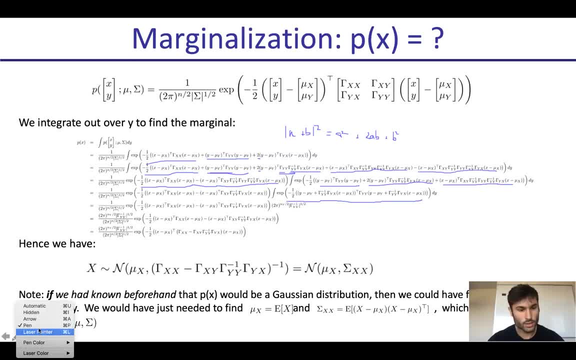 of, because this essentially so we can consider that this is the, this is the mu term of the of a Gaussian, this is the inverse of the of the quadratic, and this is again the mu term Right. so now we can just like plug in the formula. 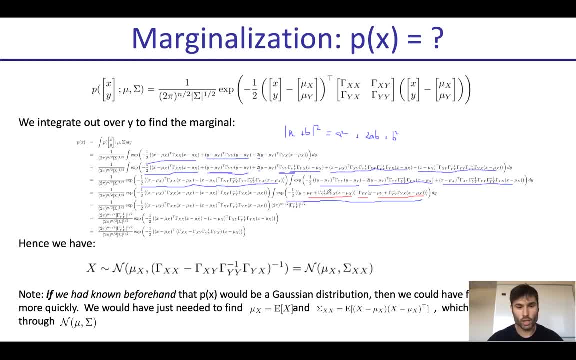 that we that we obtained for the PDF of a Gaussian and with, like some indirect manipulations, we obtain that this is the marginal of b of x. So what this will mean is this, this mu, it's the mean and this term over here is the inverse of that of the covariance. So essentially, we just have that. 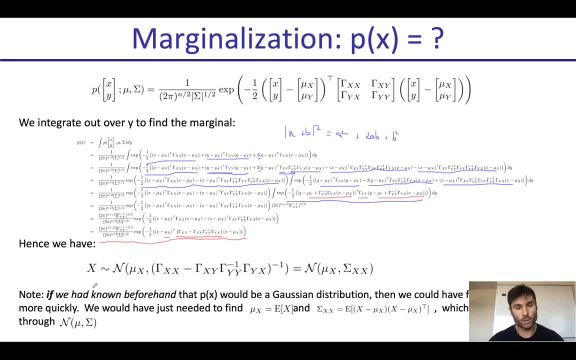 the Gaussian random. the Gaussian variable x follows a Gaussian distribution with mu and covariance matrix, which is sigma by p. We can plug in the previous relationship that we found out between the precision matrix and the covariance matrix. So we have done all these manipulations because we didn't 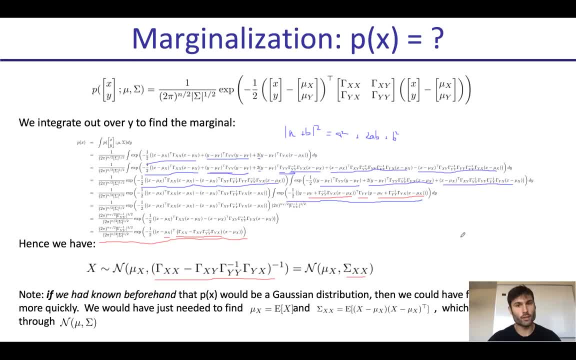 know beforehand what will be the form of the, of the marginal of x. But notice that if we had known that the p will have inner Gaussian, we could just find out the mu and sigma. So that will make our lives way easier, because we know that the covariance matrix will have inner Gaussian. So we could just find out the mu and sigma. So that will make our lives way easier, because we know that. 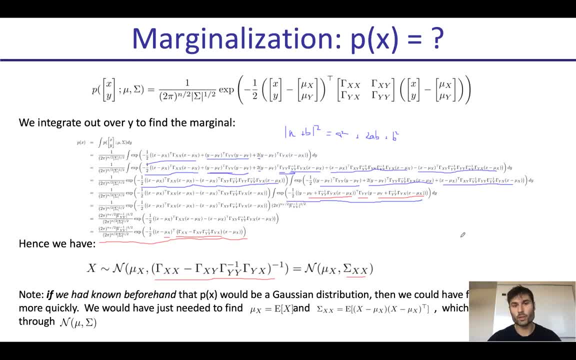 the Gaussian variable is just parametrized by the parameter mu and the parameter sigma. This is like the, the mean and the covariance. So we could just like have found out the mean and the covariance of the of the variable x in order to to find this distribution. But we assumed beforehand that we didn't know what was. 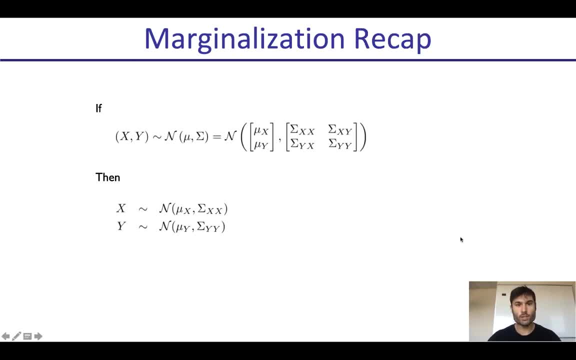 the form of p. So just a quick recap: if we have a joint distribution that follows this, like this partition variable with parameters like mu x, mu y and all the covariance terms, Marginalizing is pretty straightforward: It's just get the mu, the mu of the of the parameter x, and then the covariance of the. 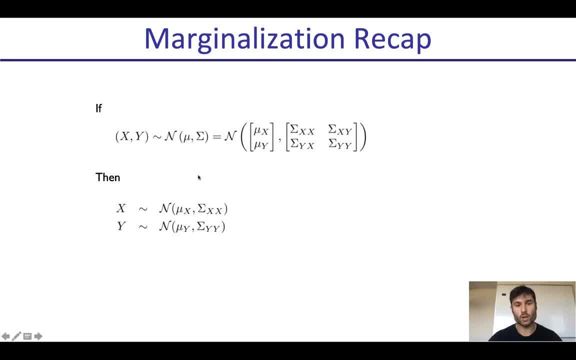 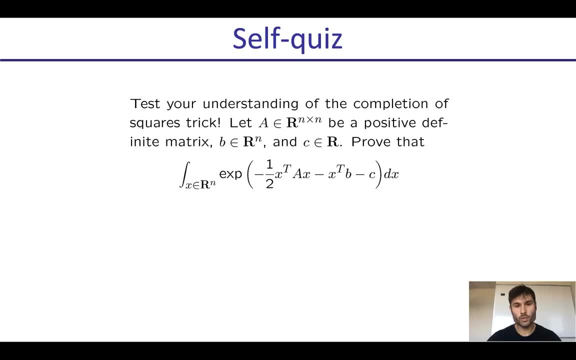 parameter x also, And the same if you do it with respect to y. So you will have to work. it would be good for you to work through all the details how to essentially do the competition of square-streak. What I essentially hinted in the, in the, in the proof before, But I just like sort of 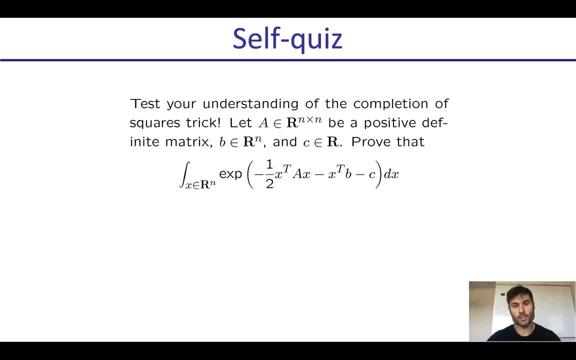 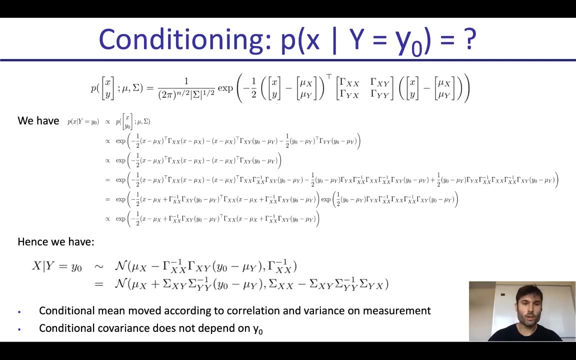 specify it for the, for this scalar case, But you should be able to work it out yourself and find out that this interval over here leads to the following result: So the other operation that we will need in order to to the to fully formulate the Kalman. 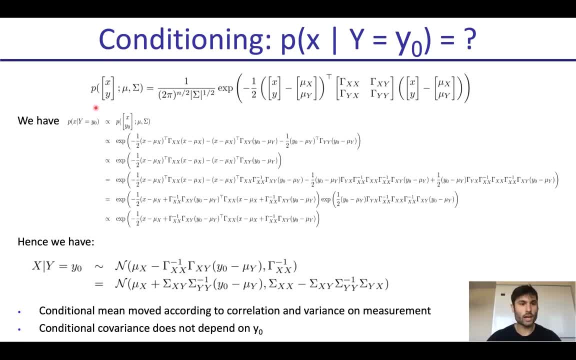 filter is conditioning. So essentially we have the the joint distribution p of x and y. If we know that the value of y is equals to this y0,, what is the value of? what's the probability distribution of x condition of y equals to this y0?? 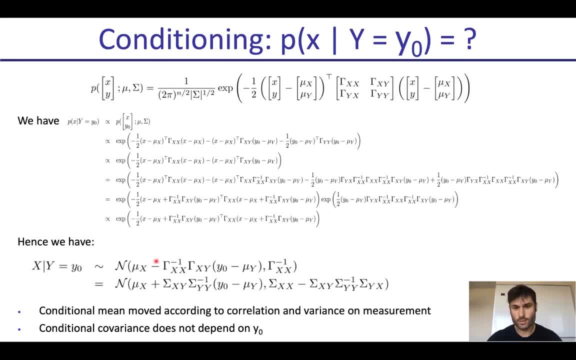 Again, we'll work more or less through this daunting math, and it's using this, the exact same tricks. So here what we're saying is: the probability of x, given y equals to y0, is proportional, and that means that it doesn't depend on x to the. 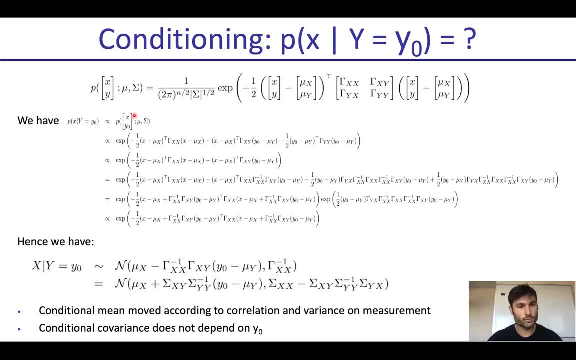 to the joint distribution of x and evaluating y to y0.. So just expanding again the, So just expanding again the, this expression, this quadratic expression, we find that it appears, these three terms, One that just depends on x, this depends on x and y0, and this just depends on y0. 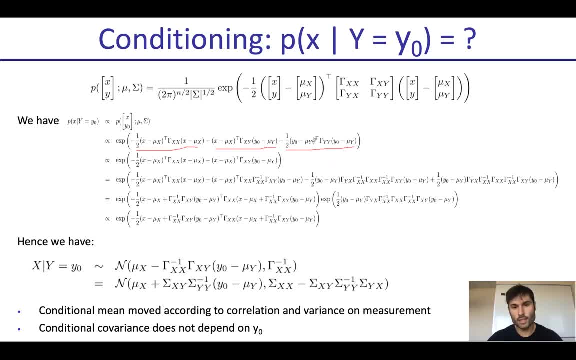 Since we're just like finding, like proportionals, and this term doesn't depend on x, we can just completely drop it off and just say like: oh, all of this is again proportional to just the terms that depend on x and the parts that depend on x. 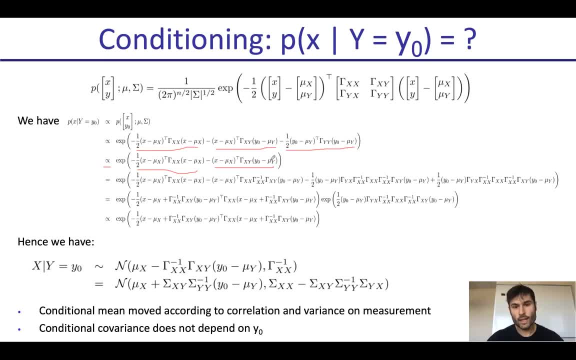 And again we can do the same. we see that this like similar to a quadratic, but not yet a quadratic. So we also, we will massage this expression by using this computation of squares trick. again, And the tricks are very similar here we'll also adding: we'll just multiply it by one and just doing. 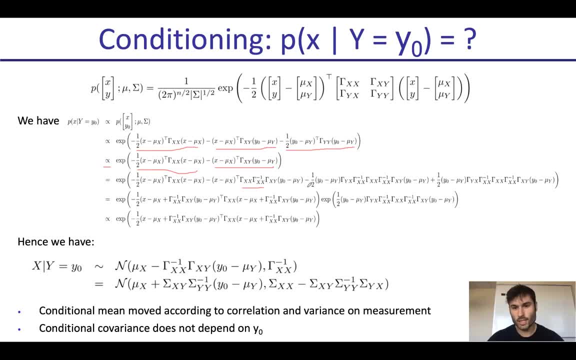 gamma xx times gamma minus one xx. and just adding and subtracting the b squared term in the computation of squares trick. So this term, again just the b squared term, doesn't depend on x, so we'll just like move it away and say it's proportional. And now the other terms over here, just like they form a quadratic. 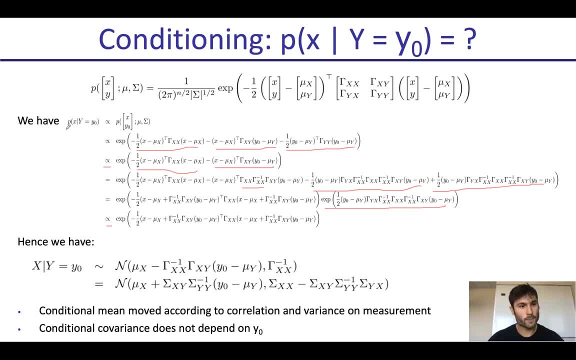 So essentially, you end up finding out that the, the conditional of x with y, equals to y0, it essentially gives this quadratic term- And this is again the Gaussian distribution- right. And now what we have instead is that the, that the mean, is given. the mu term is given by this. 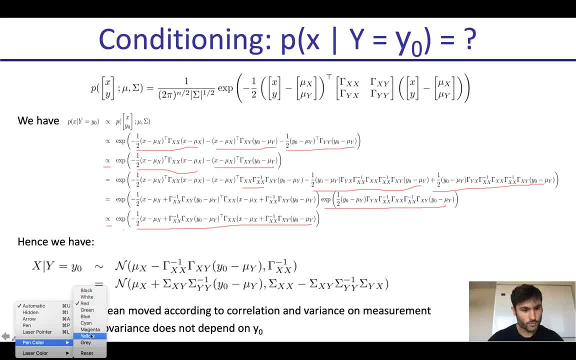 the mu will represent this term right here, and here it's missing, actually, a parenthesis. And then the inverse of the covariance will be given by that, by the precision matrix, And then here we also have the mean again. So here's what we're saying: that x conditional y equals y0. 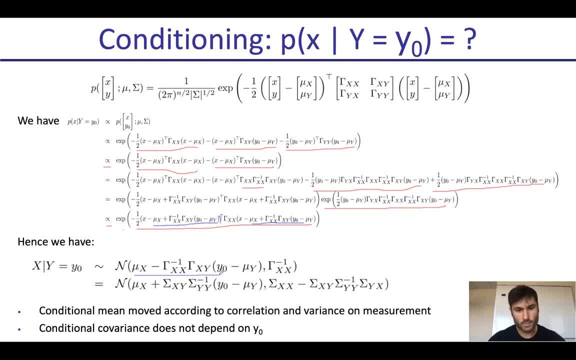 follows a Gaussian distribution That has this mean and it has. covariance equals to the inverse of the precision matrix. So now we can just write it all in terms of covariances: it's a precision matrix and this is the, the resulting Gaussian variable. 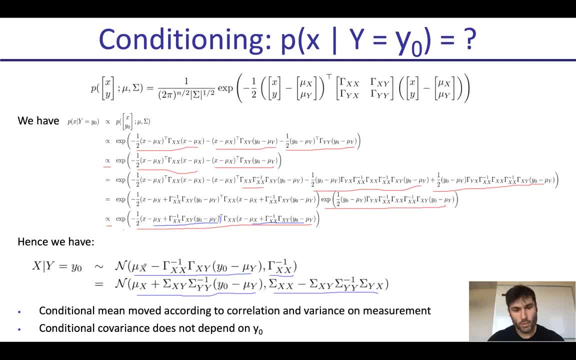 So we see that the way that the mean moves is that we have this sort of like uh, error term, Or like deviation term, That like how far is this y0 with respect to the mean, And this, like the, the correlation between x and y. 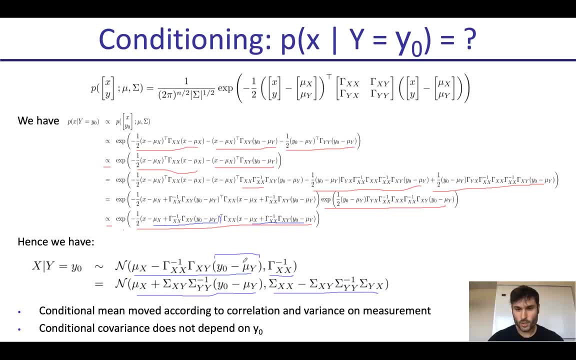 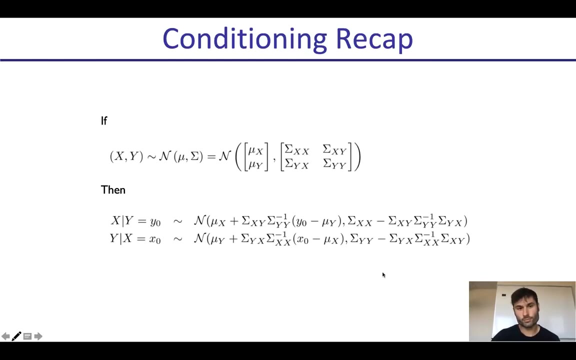 And essentially we also see that when you condition on y being equals to y0, you produce uncertainty or the variance of the system, because here we essentially from this covariance x we're just subtracting this term that is positive. So this is just a recap of the 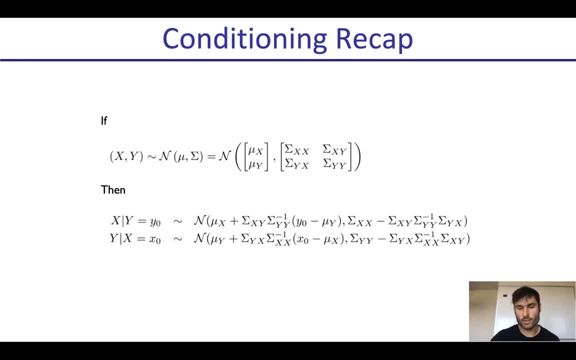 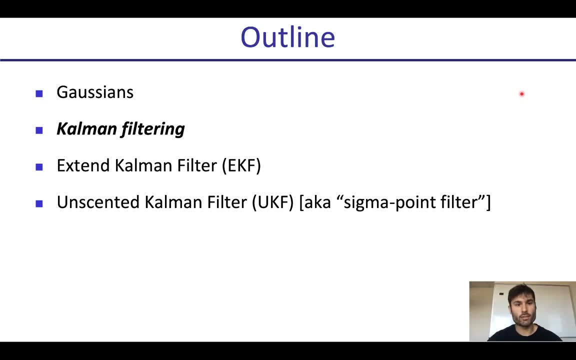 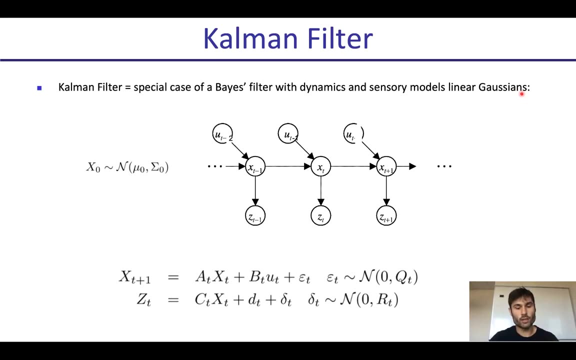 formulas that we just found out, in case you want to access it later easier. So now we'll delve into the main part of this lecture, that is, the Kalman filter. So you can consider a Kalman filter as a special case of the Bayes' rule. but when the dynamics 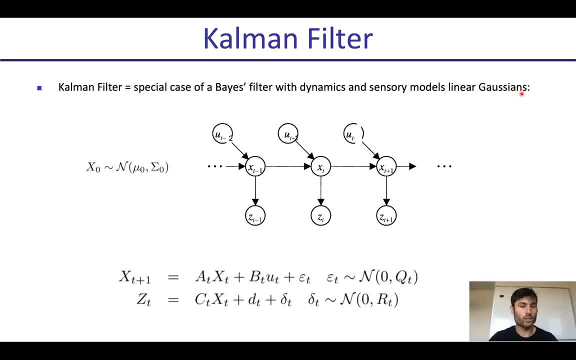 are linear and the measurements are also linear, and then if you start with a Gaussian variable and all the noise that you have in the system is also Gaussian, then what you end up having is all the variables involved are also Gaussians, and then 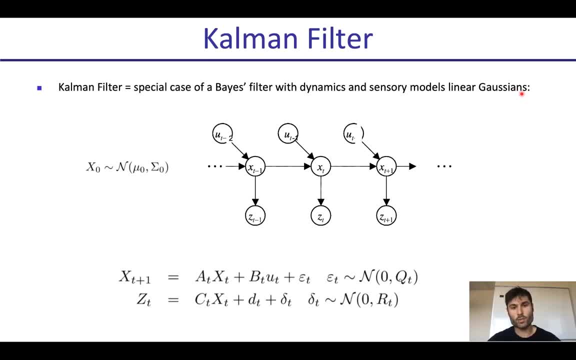 we can obtain algorithms that are much more efficiently filter and recover this state, Because the underlying assumption is that we assume that we know the first state, so this initial distribution, and then we have access to the measurements, But we don't have access to the underlying state, we don't have the x. 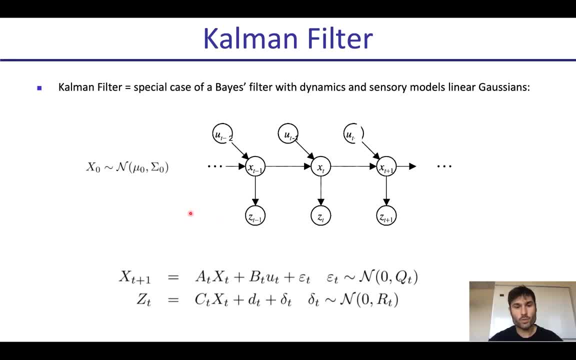 And we, given the measurements, we want to be able to recover what's a state of the system. And this is a pretty common case in robotics, where you directly don't have access to the state of the system, but you just have access to the 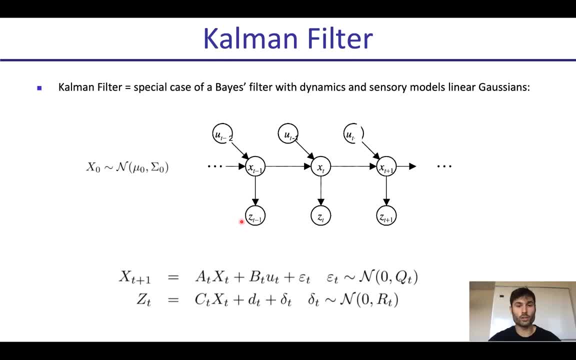 sensors that you have incorporated into your robotic system. So also what this graph is saying is that the variable xt plus one just depends on xt and ut, so there is no further dependency. so if you know xt and ut, you are able to recover the, the distribution of xt plus one, and then these zts just depends on the. 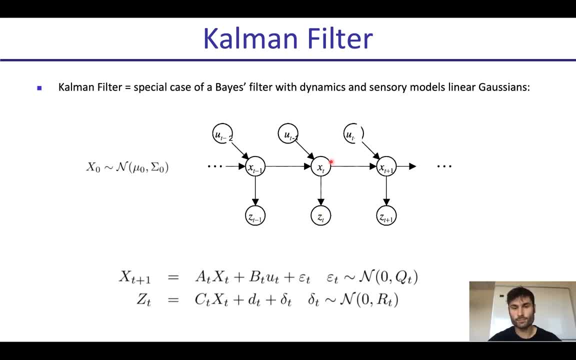 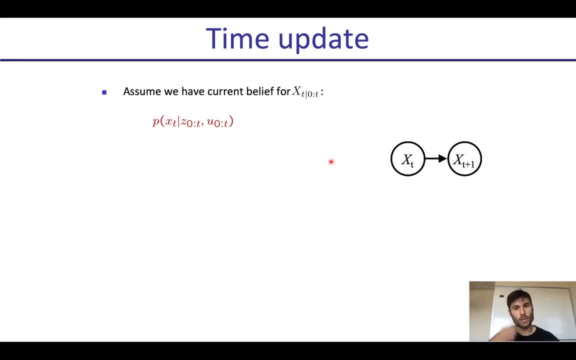 underlying state. there is no other dependency. so there are there are three updates in this uh common filter, and the first it's um the time update. so the time update is just uh obtaining the prior that you know of xt plus one given xt. so here we don't yet assume that we have observed the measurements of the sensor. 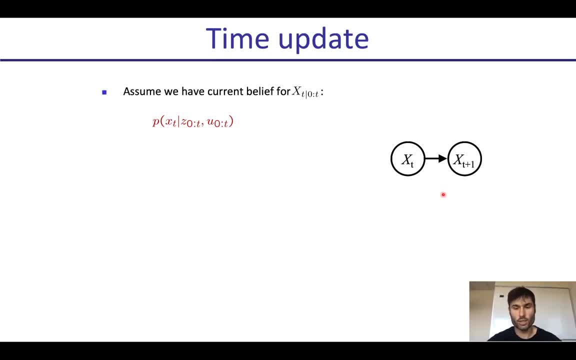 we just know that, given xt and our Dynamics model, what is the xt plus one that I predict? So here we assume that we know the probability of xt, given the previous measurements and actions, And now we want to know what will be the deduce region of xt plus one. 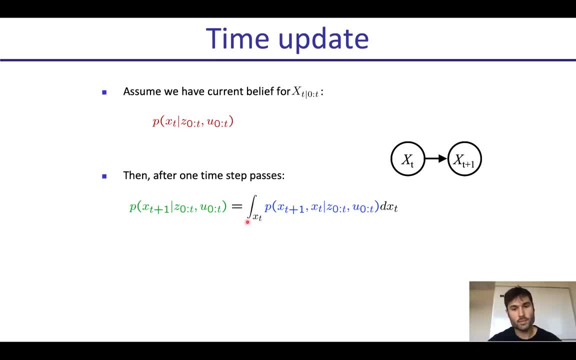 So we can just write this down as marginalizing the join of xt plus one and xt And essentially this join. we can now apply the bias rule and we could write it down as the probability of xt plus one, given xt and all the measurements and all the actions. 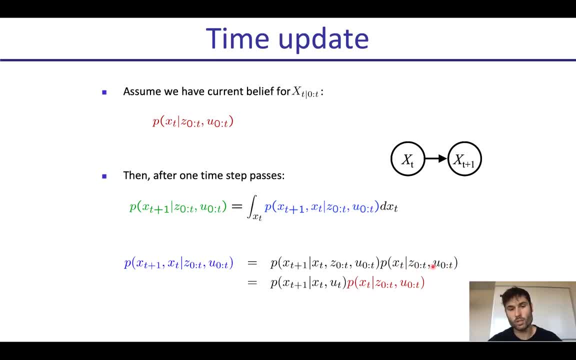 times the probability of xt, given again all the measurements and all the actions that we have here. So if we saw before in the graph, xt plus one just depends on xt and ut, So we can actually just throw away all the measurements in this term. 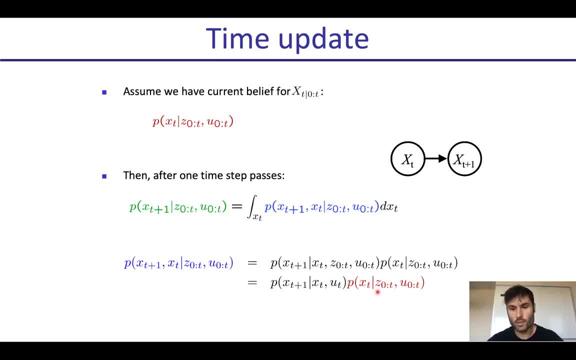 And the other component over here, this like the probability of xt given zt, a given z, of all the measurements and u. this is what we assume that we know at this current time step. So you have like this sort of like inductive assumption. 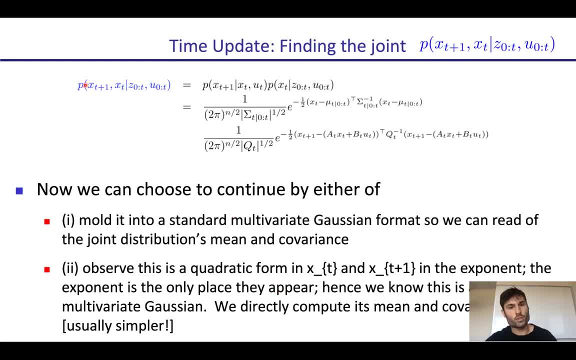 So we want to be able to find this joint. so we want to be able to find this joint and this joint distribution. And in order to find the joint distribution, we just need to find out this term over here, because we already know what's there. 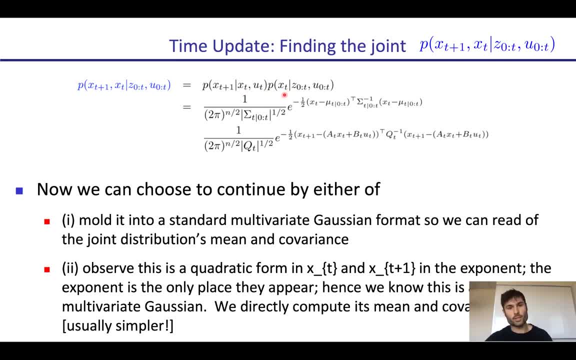 What's the? we assume that we know what's this probability of xt, given the measurements and the actions. So we can expand out this term because we have the relationship between xt and xt plus one is linear. So essentially, if we go back to the first slide, 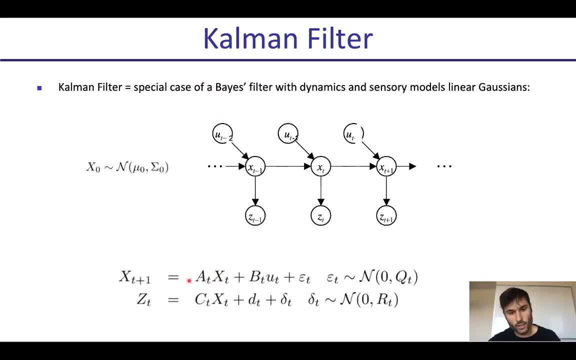 now given xt. the only randomness in xt plus one is just the noise that we incorporated. So what? this is saying? that, given xt, the random variable that xt plus one follows, it's a Gaussian variable centered in, at times xt plus b And then it has a, since there's no randomness here. 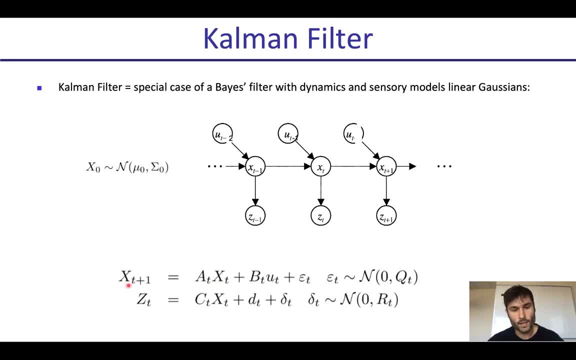 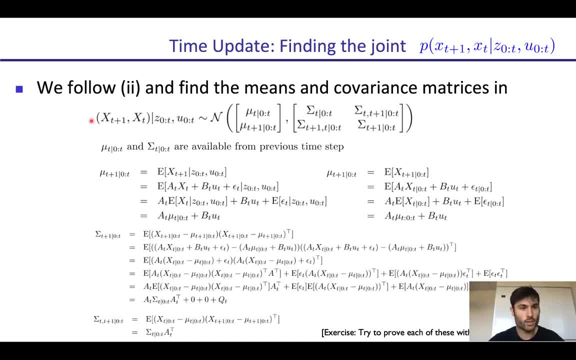 So essentially we'll have- we have a Gaussian variable that is centered in this prediction of the dynamics and has the noise qt. So here in a lot of daunting math, but it's pretty pretty, actually pretty straightforward, and you should be able to work through it without looking at this at this slide. 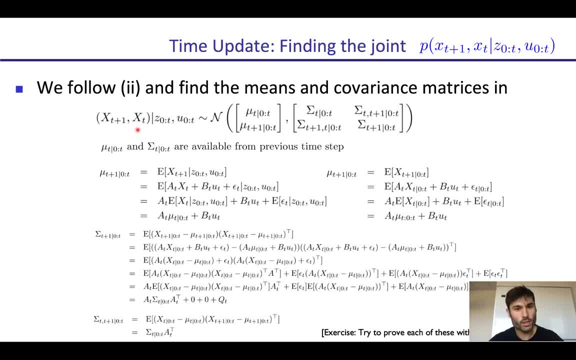